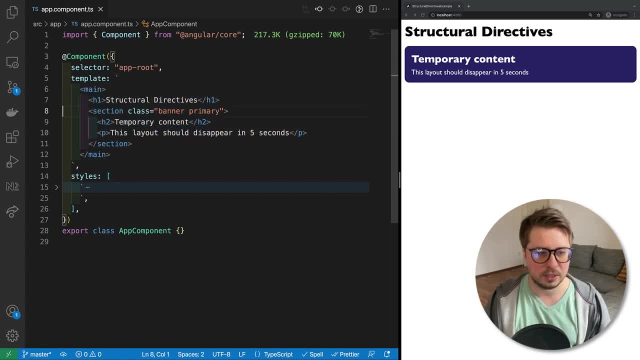 in this video, I would like to implement the next functionality, so I would like to hide some part of my template. as example, this banner after some period of time, let's say after five seconds. So it's going to be something similar to ng-if, but with some delay, and in order to implement 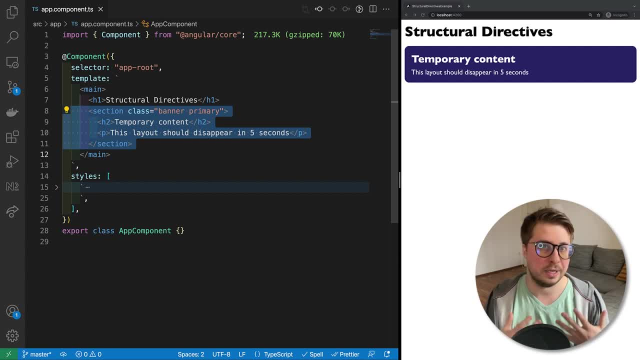 this functionality. I decided to go with structural directive because it is exactly the kind of directives which allows you to manipulate with DOM, so you can either reshape it or remove or add some templates. and it's good to encapsulate this functionality in some directive which I could reuse within my application or even extract it to the library. 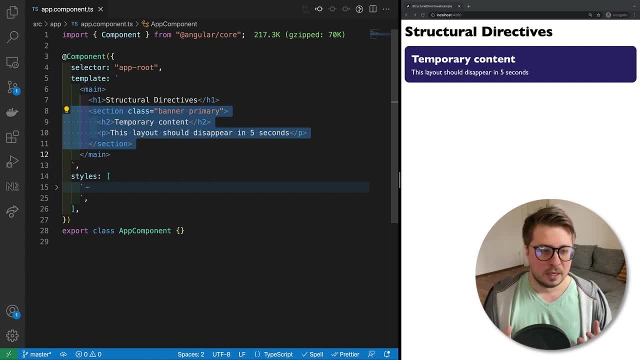 and ship to other teams. So let's get started and implement our function. So let's start with the first structural directive and in order to generate the directive, I will be using the Angular CLI, so I will type ng- generate directives, just the shortcuts g and d. 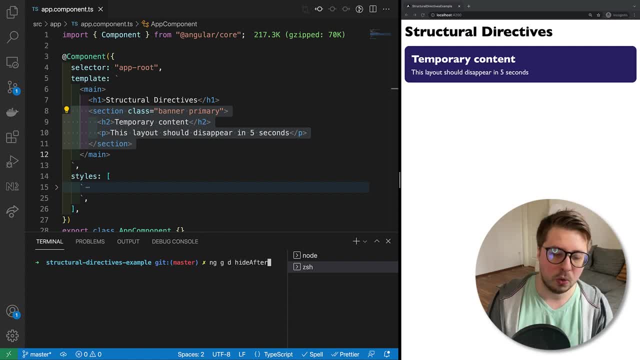 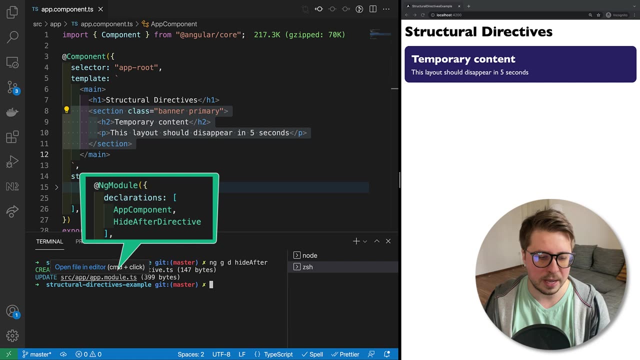 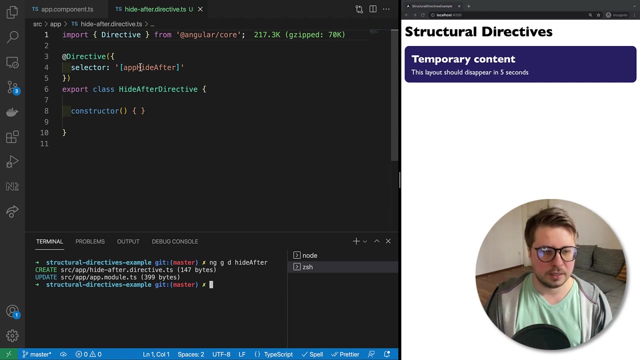 I will generate directive which called hide, after I decided to call it like that. Once I press enter, Angular CLI will generate The empty directive for me and it will add this to the declarations array inside the app model. Okay, let's jump to the directive and let's a little bit rename it. 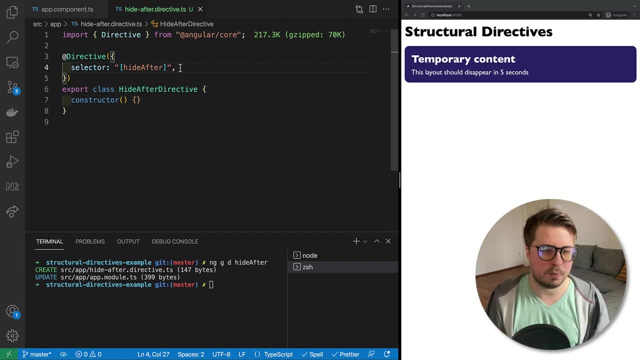 I just want to have hide after to not have this prefix. but in real applications, of course, it's good to prefix your application directives, components in order to avoid the collision with components and directives. So let's just say that we will be using the same directive for the third party libraries. 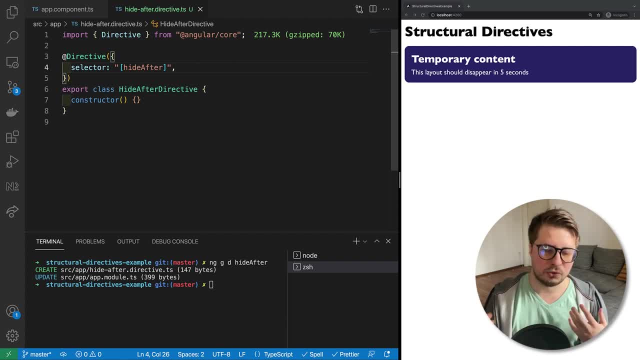 But okay, and at this point, as you can see, there's no difference between structural and attribute directives at all. They look the same. The difference is obviously in the implementation and in the way how we attach this directive. If you remember attribute directive, you attach like this: 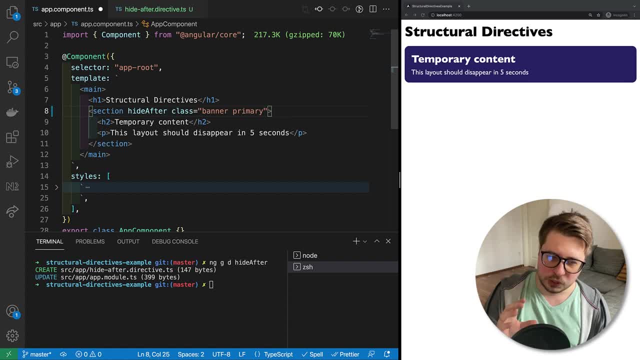 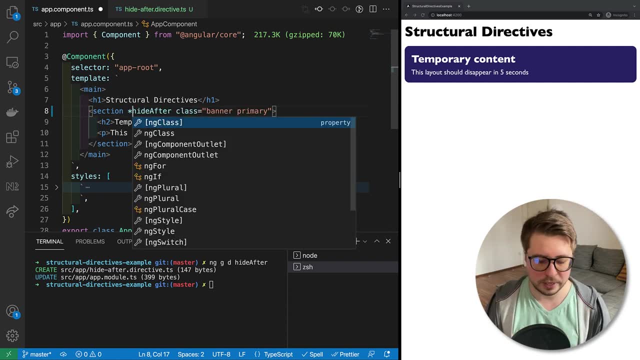 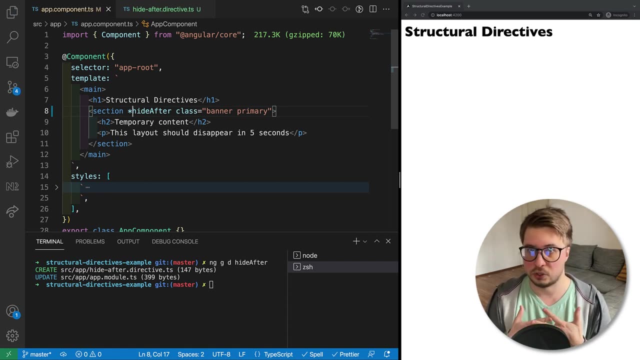 Add it here and you are ready to go With structural directives. you have to add the asterisk in front of the directive name. So, doing this, you use this directive as a structural directive And you can see the first like result. our banner has disappeared and it might be quite. 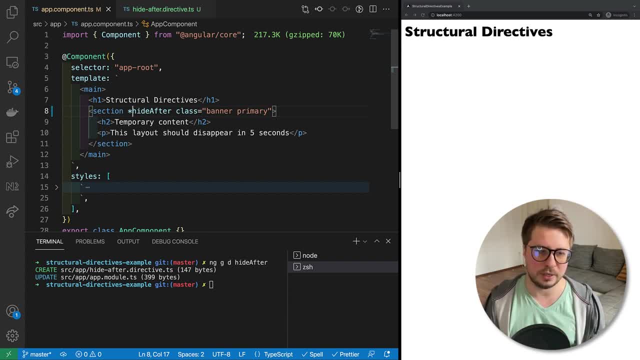 strange behavior Like why, When we attach the empty structural directive, it disappears. The thing is that this asterisk, it is a syntax sugar which wraps under the hood our HTML, where we attach this directive into ngTemplate. So basically it looks like this: 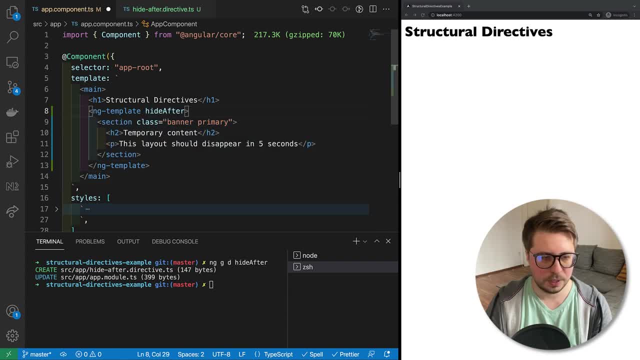 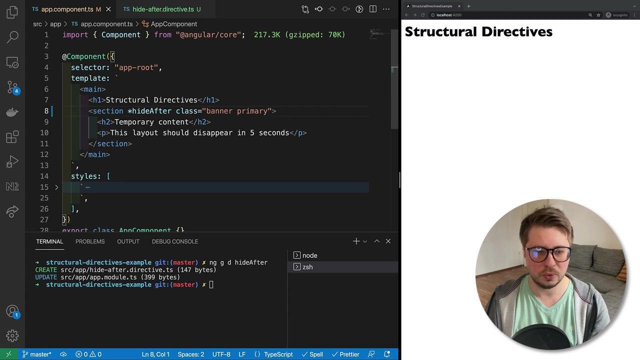 Here we go, move it inside here And, as you may know, ngTemplates are lazy, So we have to explicitly instruct Angular to render them, And that's why we see actually nothing on our screen. So let's revert it back and I will show you how to actually render this template in our 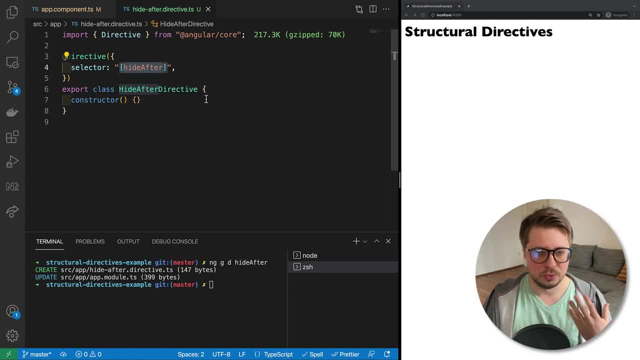 view. In order to render it, we have to go to our directive and we have to inject two things: We have to inject Reference to the container where we're going to render the template, and we have to inject the reference to the template itself. 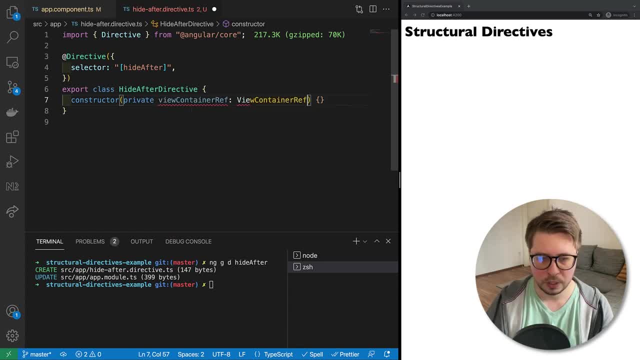 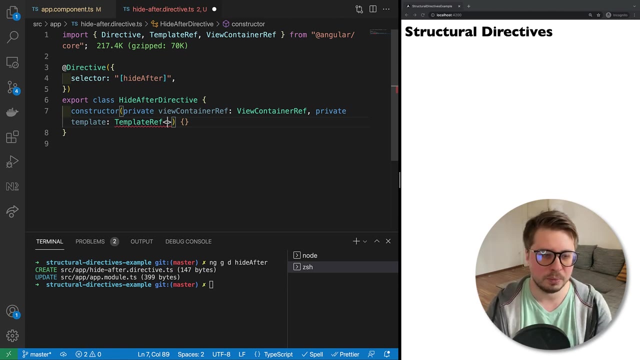 This is how we can do it. Here I inject view container ref. This is where we're going to render it, And now I want to inject the template and template ref. It's a generic, so we have to define the type of the template ref. 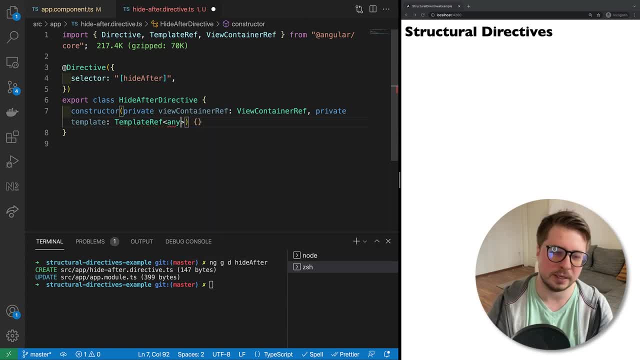 But in this case It will be okay if we say that the type is any Cool, So let's save it. And the second step is actually we have to instruct the Angular to render our injected template in the injected view container ref. And I will do it inside ngOnInit lifecycle hook. 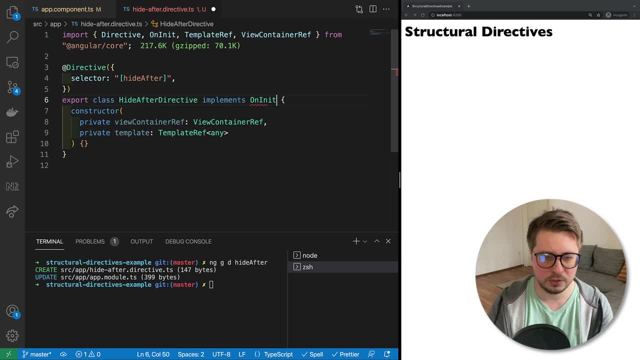 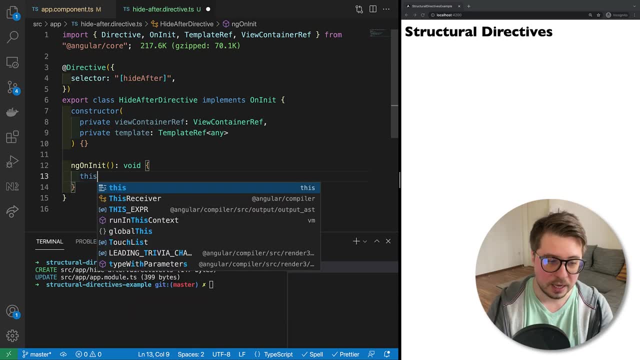 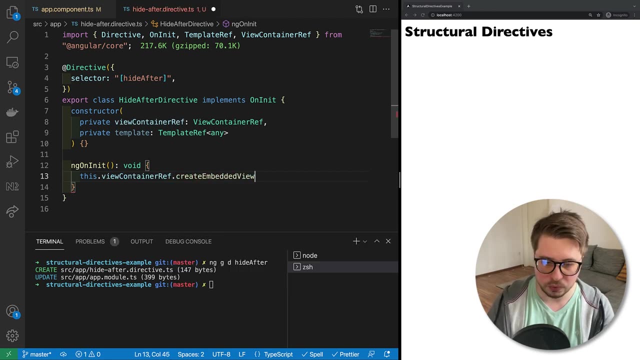 So let's implement this interface, And here below I'm going to create My ngOnInit method and inside I say that view container ref should create embedded view, And as an argument for this method, we have to provide our template. Cool, And now, if I save it, you can see that our banner got back. 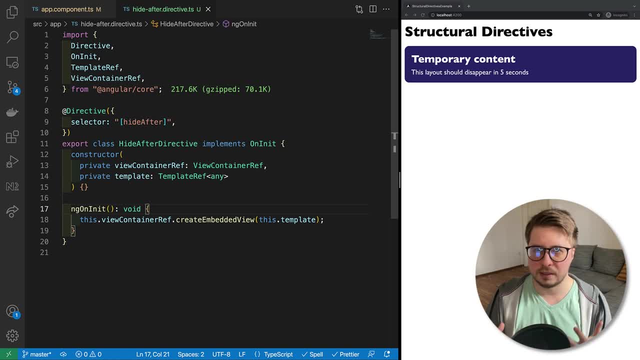 All right. The next thing we have to do is to provide, somehow, values To our template. So we have to configure the directive to hide the view after some period of time, And we have to do it via inputs, Right, So let's implement our input. 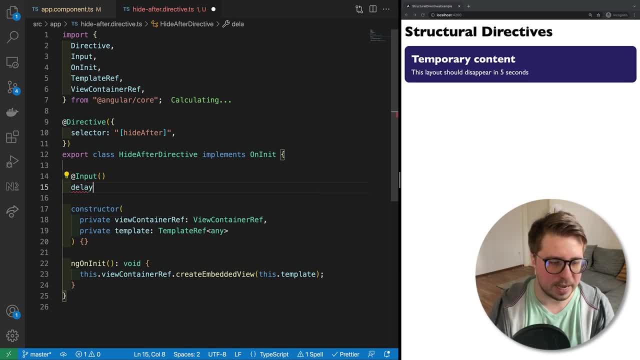 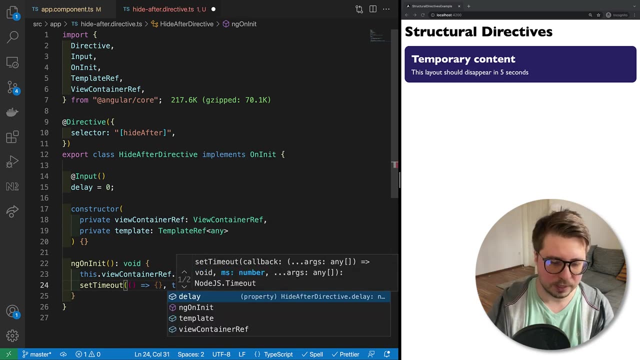 And I'm going to say that this is the input name delay, Which is zero by default, And there, inside ngOnInit, We would like to have Something like this And here Something like this Like set timeout And after some delay, 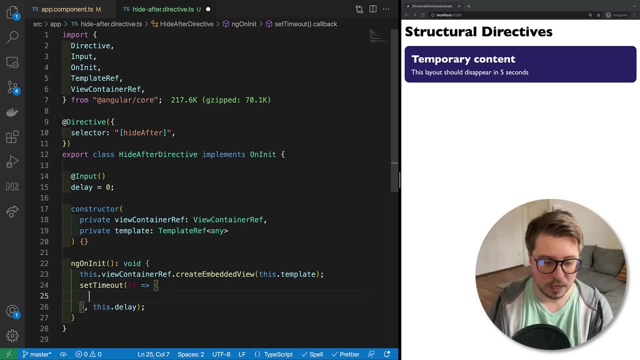 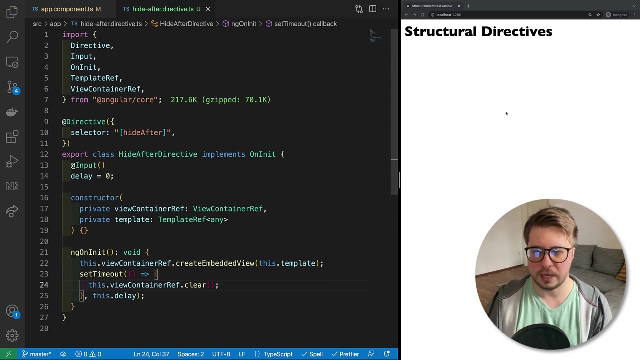 Yeah, Which we're going to define via input. We have to remove this banner And in order to clean up the view container ref, We have to call the method clear. So clear will remove all rendered templates inside this view container ref. And now, if we save it, 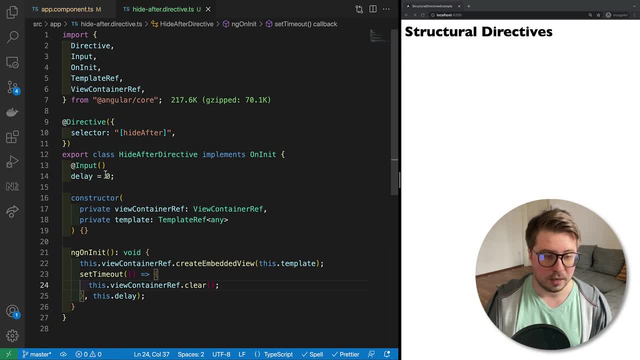 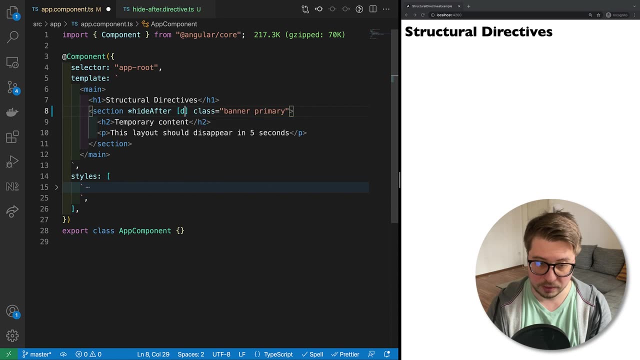 We will see that banner again disappeared Because we have zero delay And it will be immediately disappeared. So that's fine, But let's try to provide some input To change the delay And if you try to apply it like this, You will get an error. 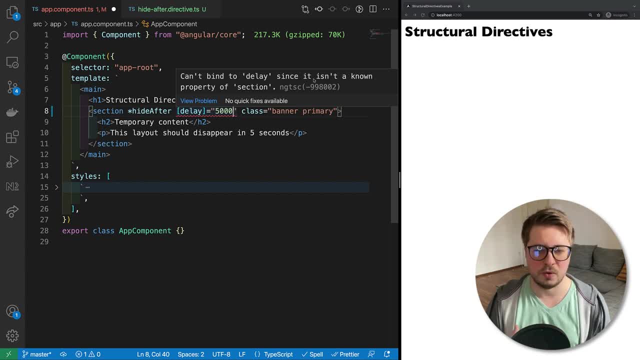 And it says that we cannot buy delay Since it is not a known property of the section. And this is only the first difference with the attribute directives. You cannot provide inputs like this. And do you know why? Try to guess it. This is because what I showed you before 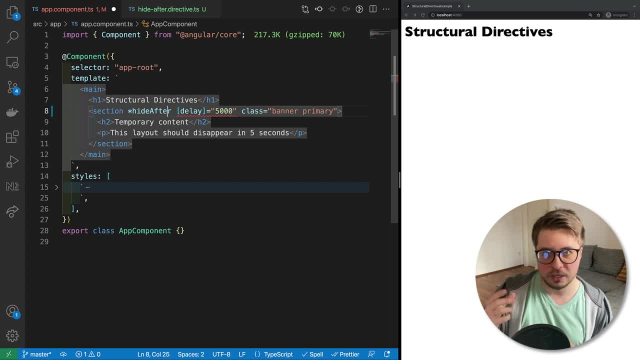 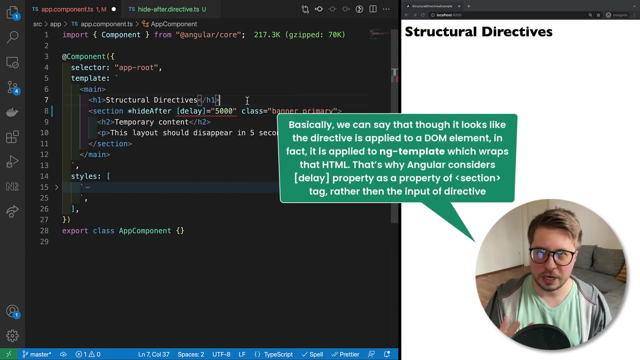 That structural directives. They are wrapping it into template, So Angular tries to resolve this input As a property of the section, Which doesn't obviously exist, And if you use the notation with ngTemplate, It would work, As you can see. 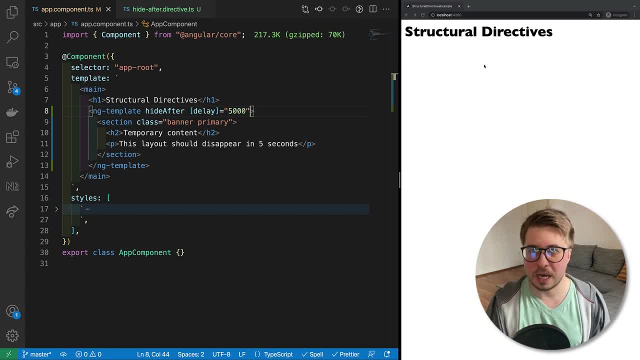 We have the banner And then after some time it disappears- After 5 seconds, which I defined, And if you want to use inputs with this asterisk notation, You have to use the special syntax for those directives. So let's revert It back. 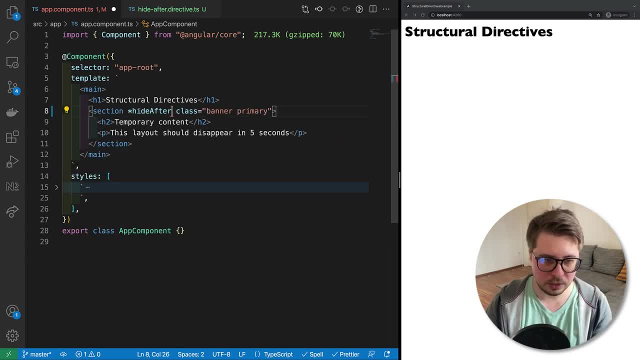 And for input values. We are not going to use this notation, But input values for this kind of directives Are provided inside these quotes. So I would like to have the next syntax. I want to provide it just like that. So, height after 5000 milliseconds. 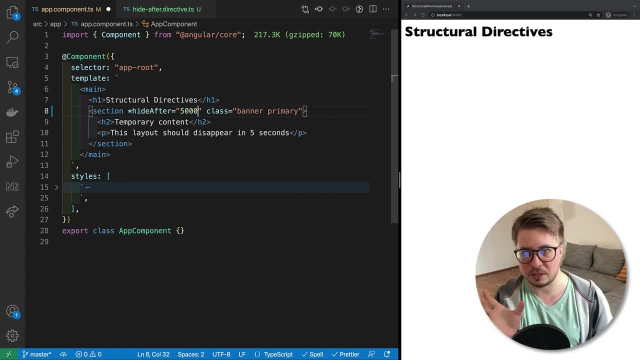 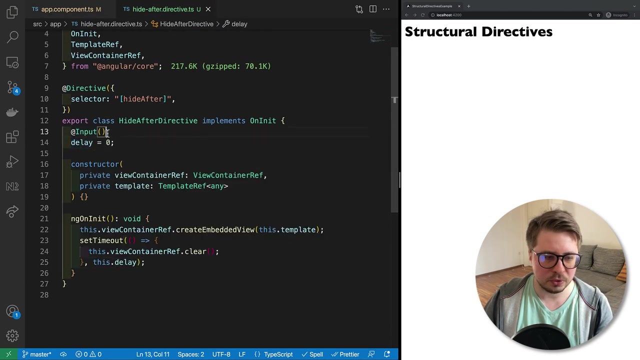 It is easy to read And it's quite short notation. So if I want to achieve It like this, I have to name my input Exactly the same way As the prefix of the directive, So I need to copy it And then I have to rename my input. 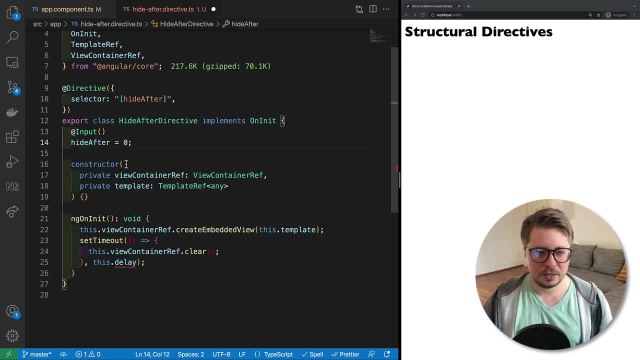 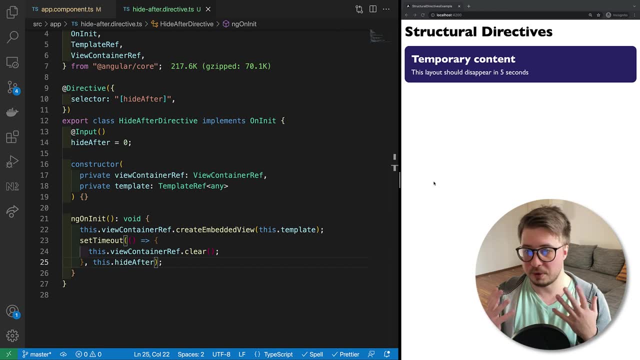 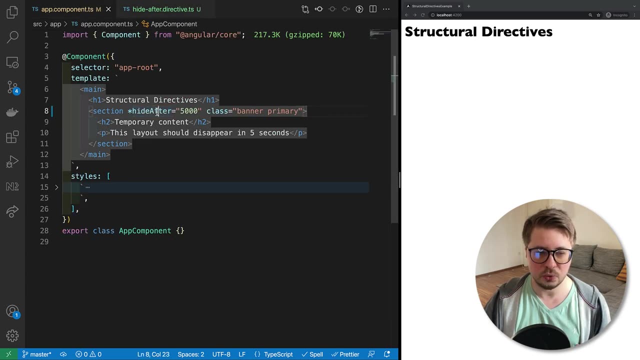 To this notation And then, if I save it- And of course I will update it here- It will be working fine, Because if you have input with the same name as a selector, You can use this notation. Okay, I hope it is clear. 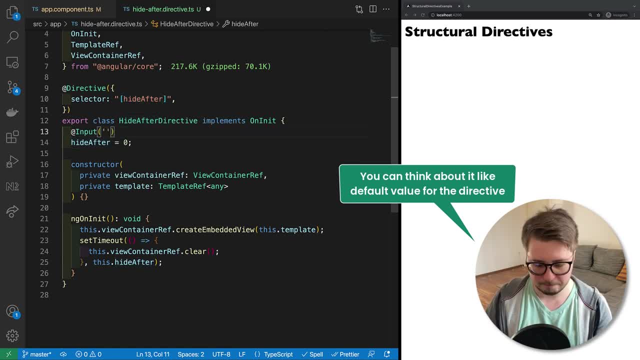 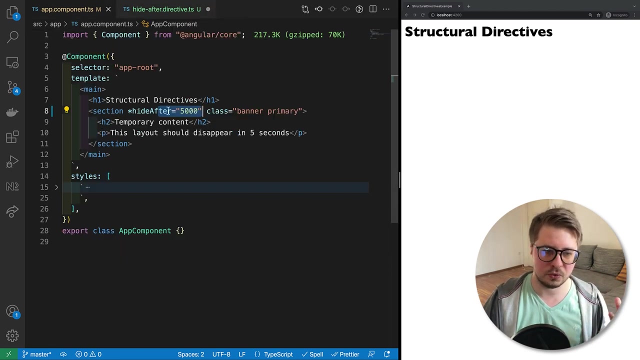 Also. alternatively, You can provide it here Like height after, But then you could just rename it Like this. So this is string inside the input. This is how It describes your API. This is how the user of this directive interacts with. 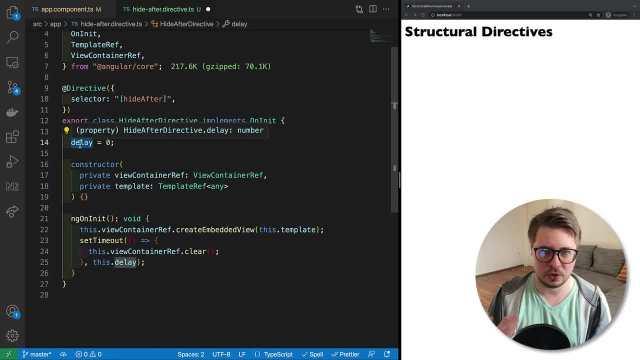 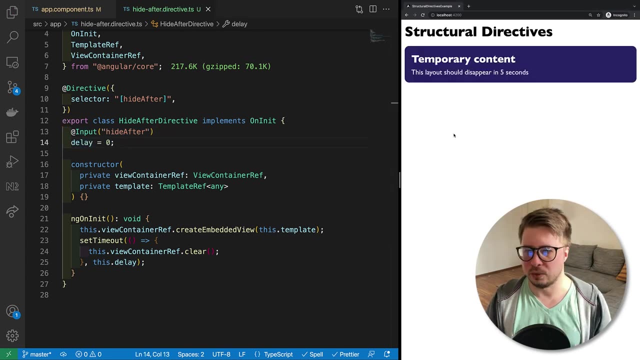 And this is just for internal implementation. So I will leave it as it is, Because in context of the class itself, I think delay has a better name Rather than height after. So I will leave it as it is. Alright cool, So our directive is working. 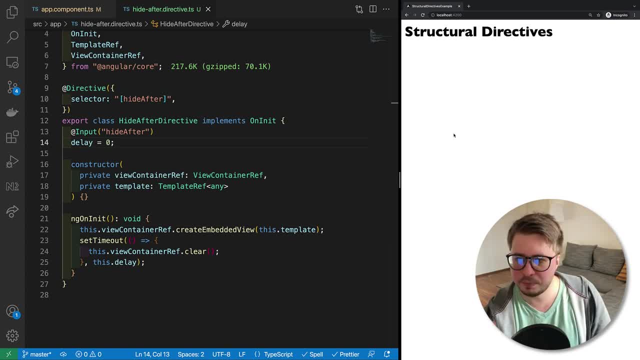 But check this out: After 5 seconds My banner disappeared And I see nothing. But what if I would like to render some Another template instead of it? Right, Some placeholder Like here was rendered banner or whatever, And I want to have it somehow similar to ng-if. 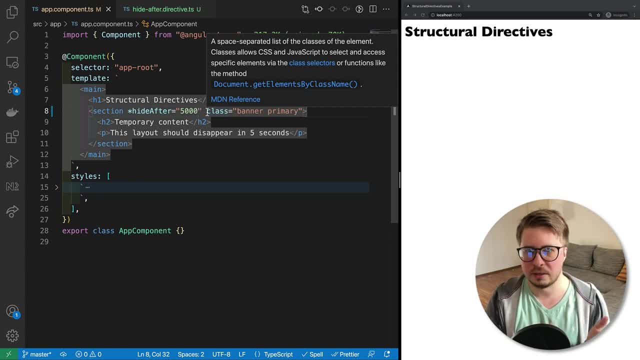 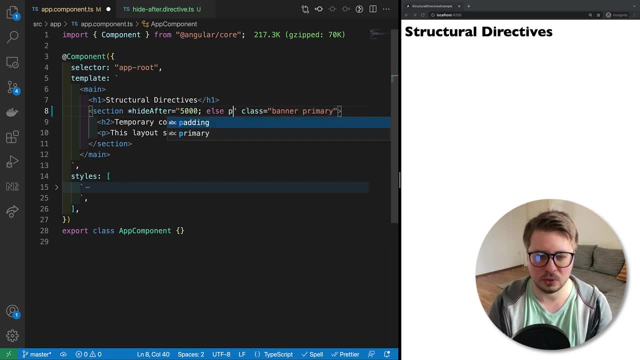 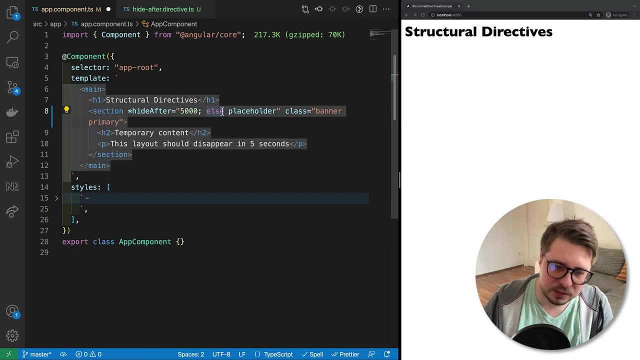 If you know that we can do ng-if And then we can do something like else And render some placeholder- In this case This else, Or in our case, let's rename it- to, then, And this, then, is just another input for the directive. 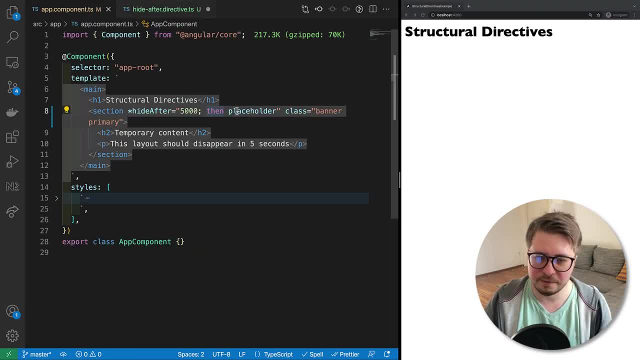 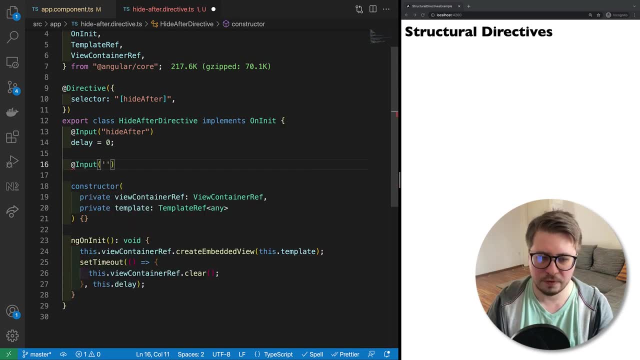 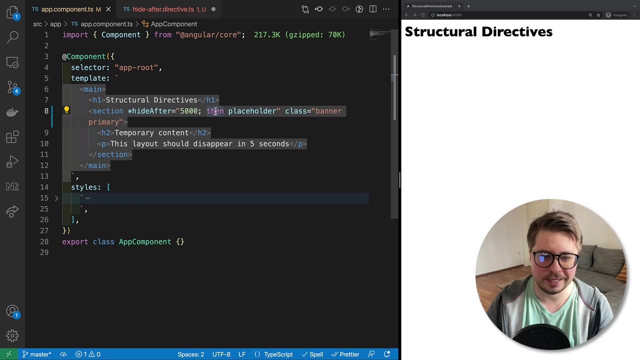 And if we want to get this value- Value for then input- We have to obviously create a new one. And here, very important, You have to add the prefix of the directive, So height after, And then with the camel case You have to attach this, then word: 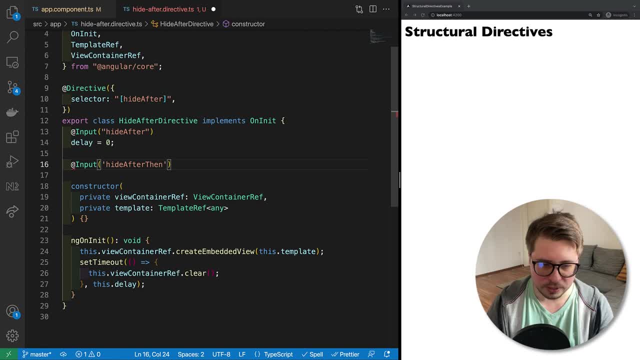 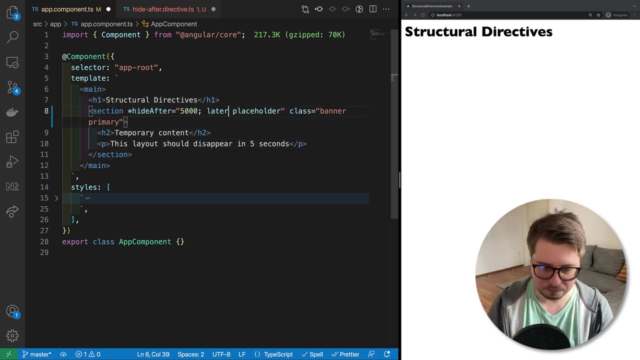 So like that. Of course, if you want to have another keyword, Let's say later as example, Then you can name it like this, But then you have to rename it Like that, Okay, So I hope it is clear, But for my case I think then sounds better. 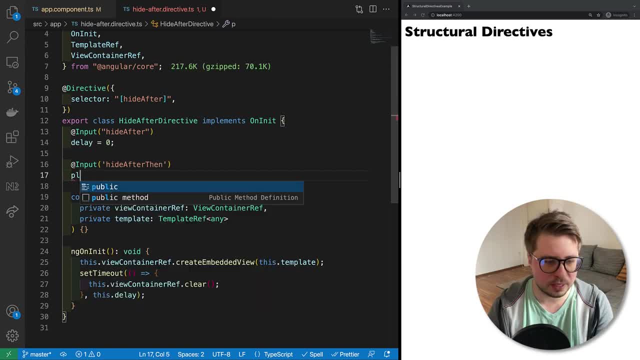 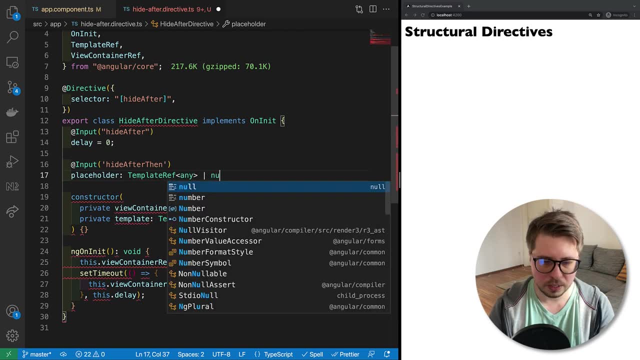 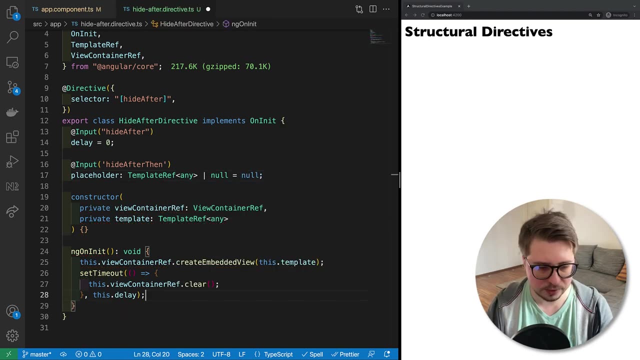 So I will rename it. And then I say that it is a placeholder Where the type either template, ref of any, Or it could be null, And by default it's going to be null. And now, inside our setTimeout, I have to, once I clear my view. 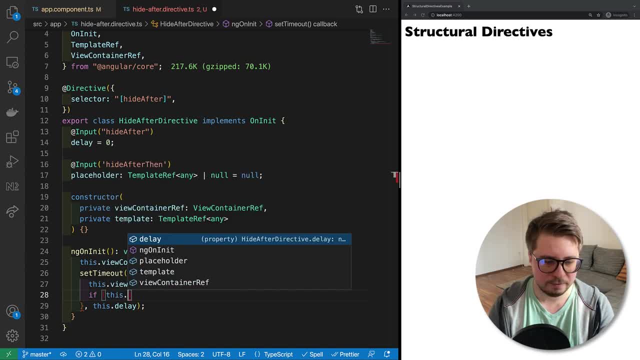 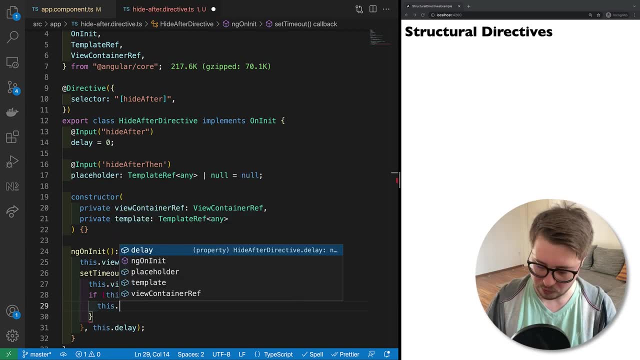 I have to check if we have placeholder. If it's not null, Then we have to render it. And the way we render it We already know. We just have to create embedded view And then we have to provide our placeholder. As easy as that. 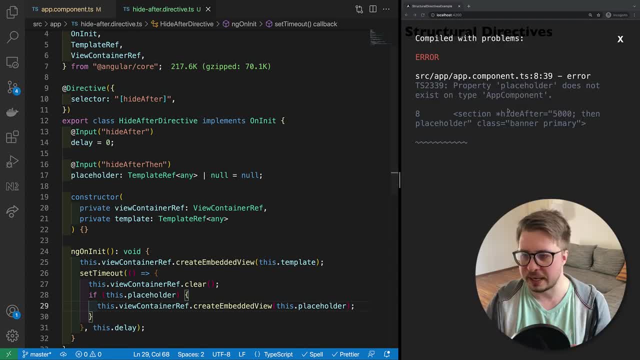 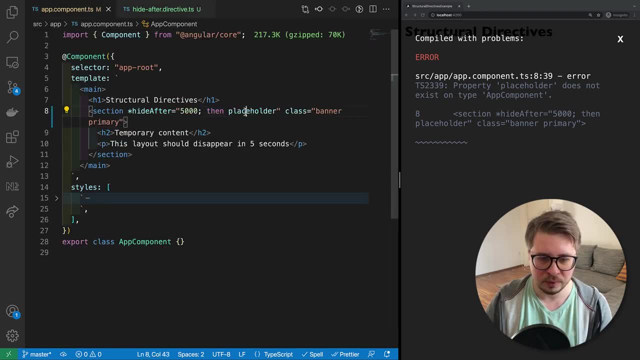 And now, if we save it, We will get an error, Of course, Because we don't provide a placeholder yet. We have to Like. this placeholder has no reference inside our template, So we have to create one. I will say So. this section will be rendered instead of our content. 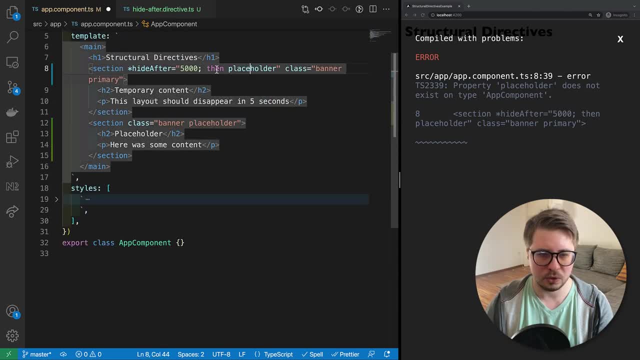 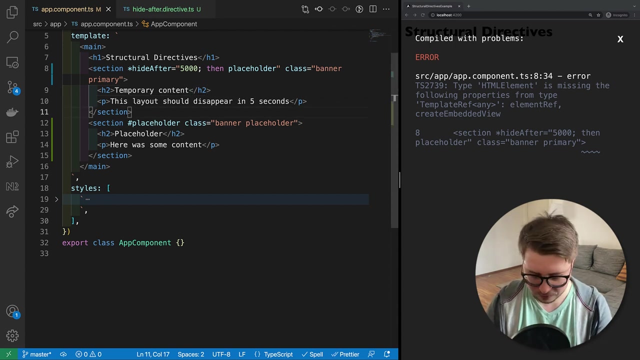 And in order to assign this placeholder to then, We have to create a template Variable Like that. So this template reference will be Eventually the input for our then input. And now, if I save it, Nothing happened. Sorry, It's my bad. 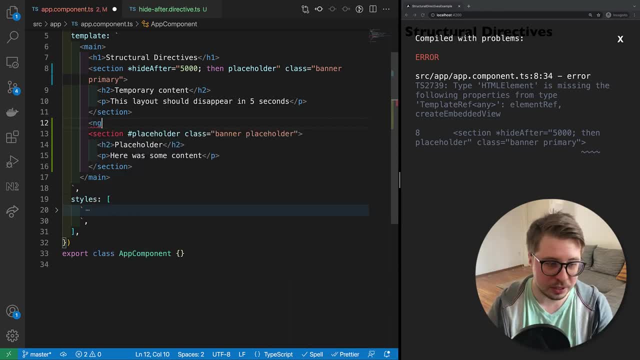 We have to provide the ngTemplate, Not the HTML element, And then create reference Not to the HTML element But To the template, And then I can Copy This Template And Paste it inside the ngTemplate. 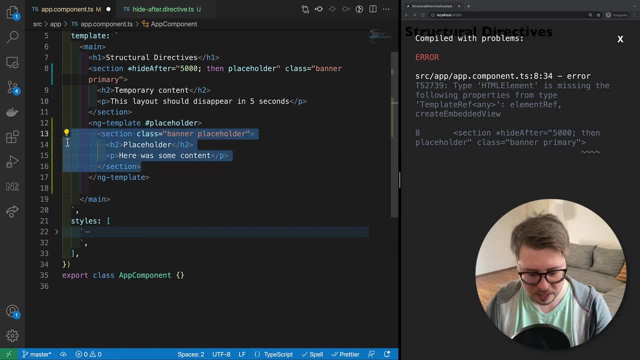 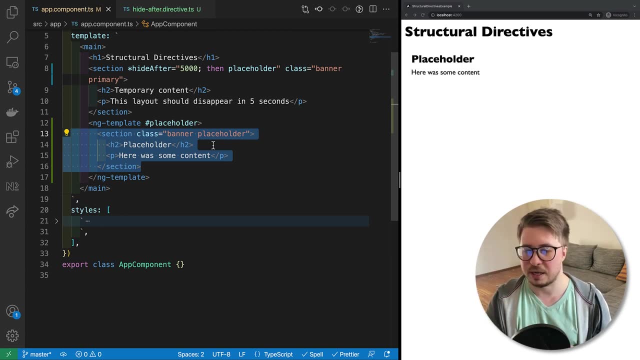 So Here we go And now, Once we save it, You can see Banner. Five seconds Past And We have the Placeholder Instead Of Our First Banner. And Though I Showed 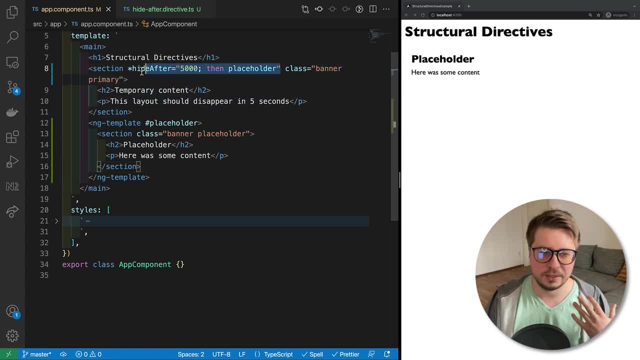 You Very Basic Features Of This Microsyntax For Structural Directive. Check out How Cool And Clean Way You Can Already Implement Some Features Like Our As. 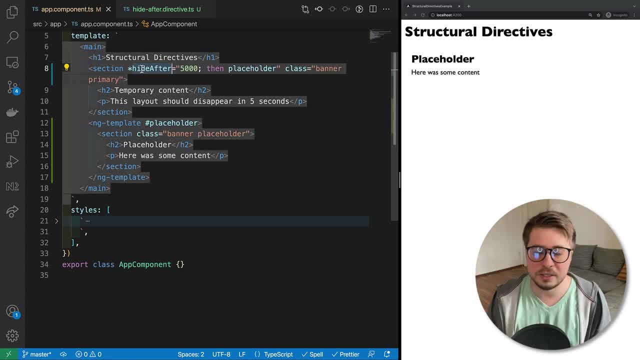 Example. It Is Very Easy To Take This Directive And Apply To Another HTML Snippet And It Will Just Work. Some Of You Who More 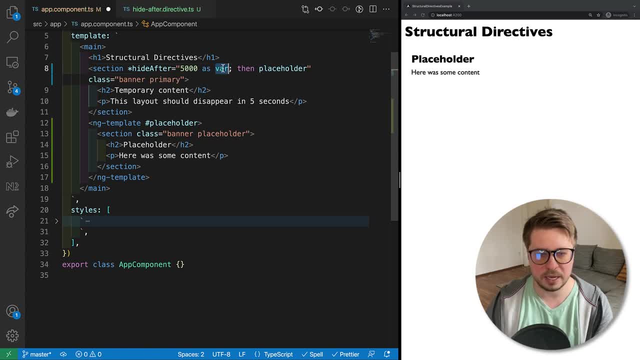 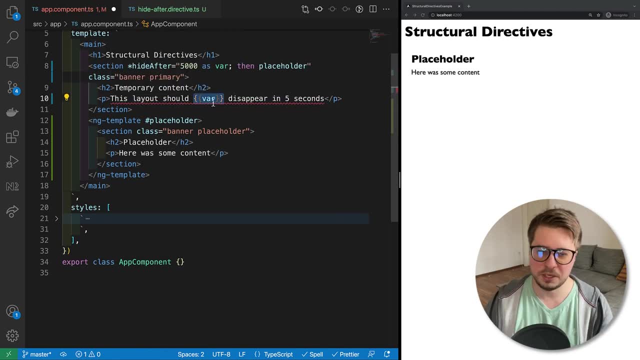 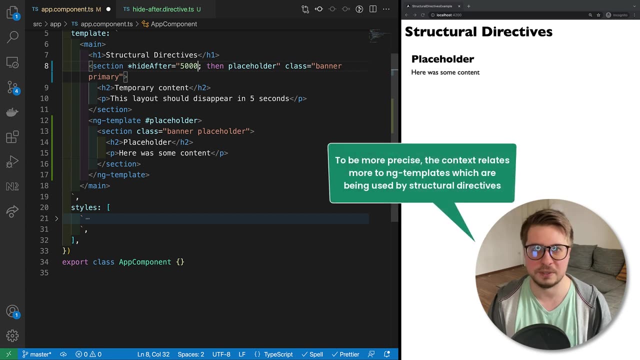 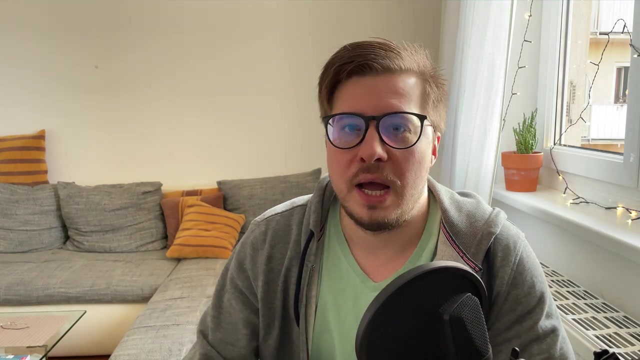 Experienced With Structural Directives. You May Have A Template Like That. In Our Case, It Will Not Work. It Will Require A Bit More Advanced.